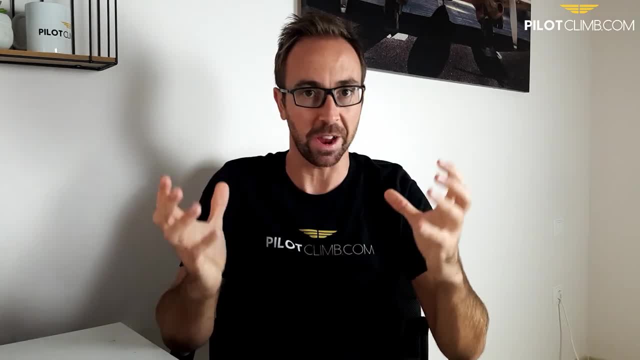 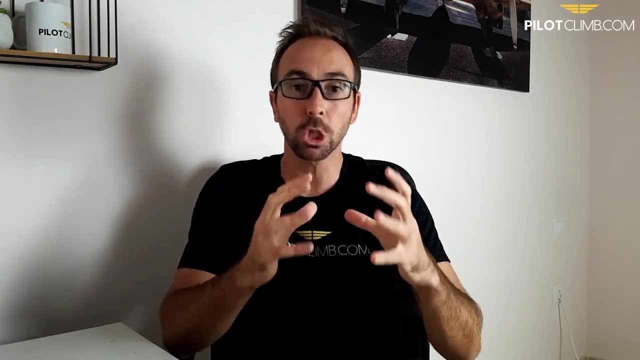 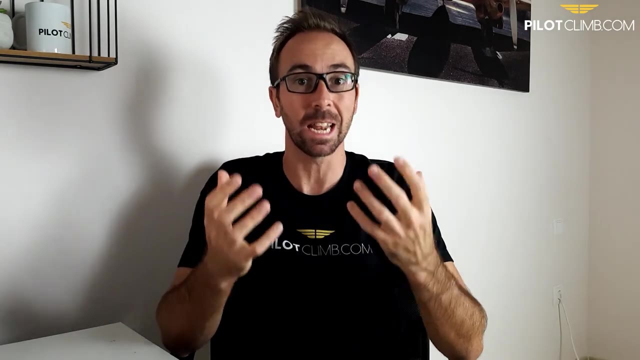 have a different characteristics compared to the surrounding air. they might be colder, they might be warmer, so they might be less dense, more dense, so heavier or lighter. normally, a mass of air that is warmer than the surrounding air, okay, is less dense, thus is lighter. so a mass of air, let's, let's imagine like: 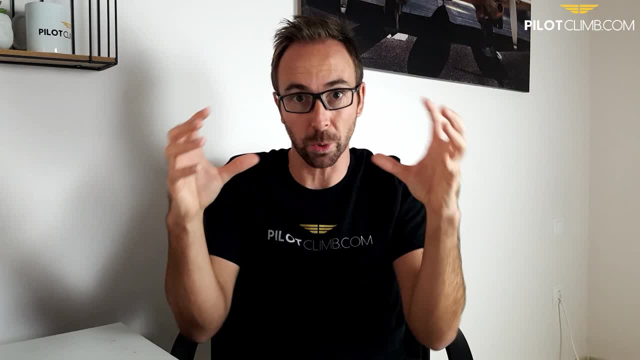 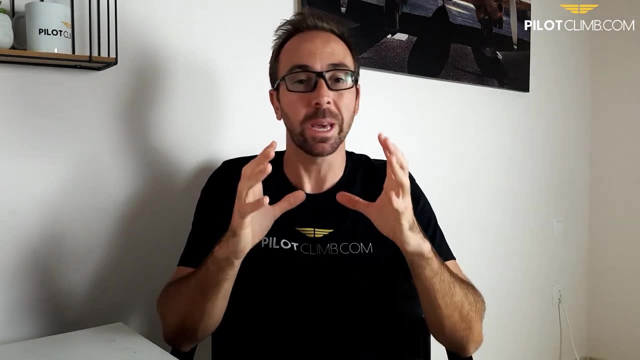 a bubble, okay, that is warmer than the surrounding air has the tendency to rise, okay. so, in order to understand what it, what is this? let's jump into the white board and let's make some examples by looking at the white board in here. okay, I, I, I. 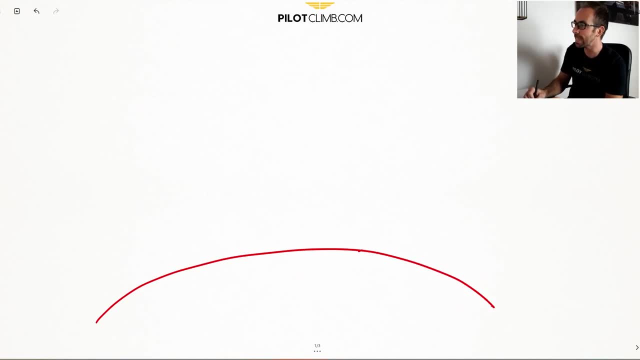 I, I'm gonna draw the the air surface, okay, and let's say, in this case, we've got water in here, so you have, let's say, the sea, all right, and then you have a road that is next to the sea. okay, so this is the air surface, and what happens is that 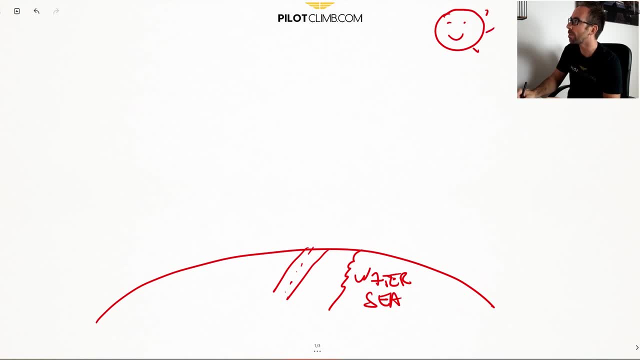 the Sun normally. okay, this is a very nice Sun. okay, sorry for my drawing. okay, anyway, the Sun will warm up the water and the air surface in general, and then the air surface will actually release this heat, this heat energy in the air- air. thus the air that is on top of the earth's surface will warm up. 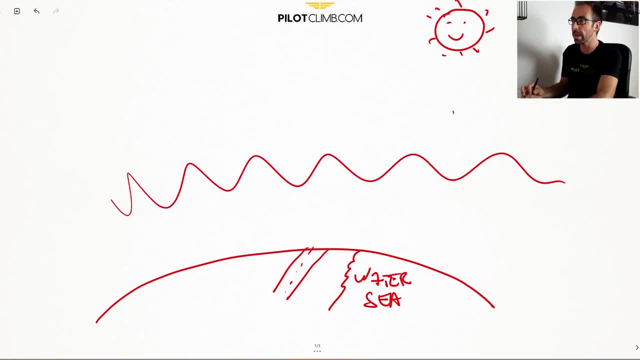 That's how, actually, we warm up the atmosphere. however, as you can already see, what happens is that if the sun will warm up the water and the asphalt at the same time, what will happen is that the asphalt is going to have a higher temperature compared to the water. 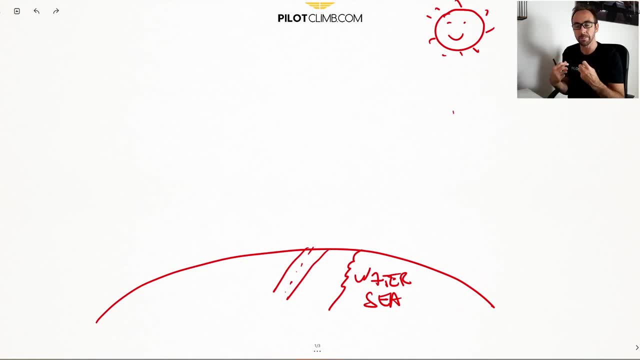 because the water has a tendency to absorb more heat and the asphalt won't absorb that much of it, so it will warm up very quickly. So what will happen is that the air on top of the sea will be colder compared to the air on top of the asphalt, on top of the road. 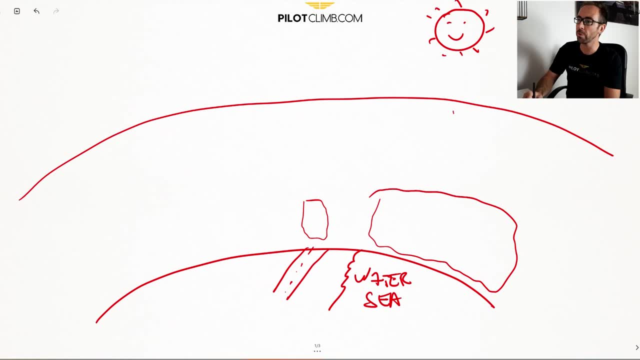 So, as you can see already- and this is the atmosphere, as you can see, we've got the atmosphere in this example. we have a mass of air on top of the asphalt, which is warmer, and then we have a mass of air on top of the water, which is colder than the mass of air. 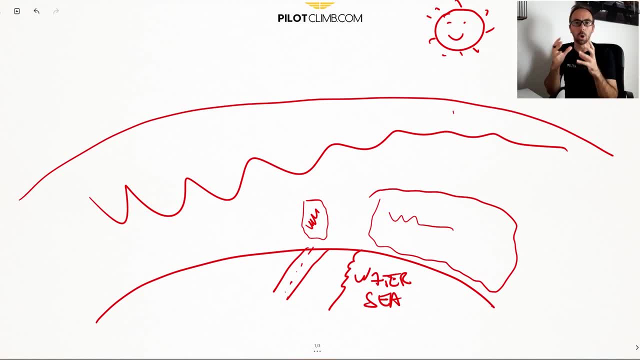 on top of the asphalt. So, in order, Why am I telling you all of this? Because it is very important to understand that the atmosphere is not a constant. nice mass of air, huge mass of air. it is not like that. The atmosphere is composed by colder mass of air, warmer mass of air. they have different. 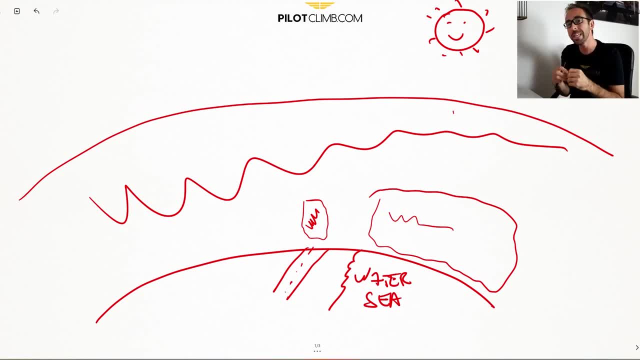 densities and so on. So you need to really understand that within the atmosphere you have different air masses and different compositions of humidity, density, temperature and so on. So now that this is clear, we can actually talk about something very important. I made already a separate video where I talk about the environmental lapse rate, the dry 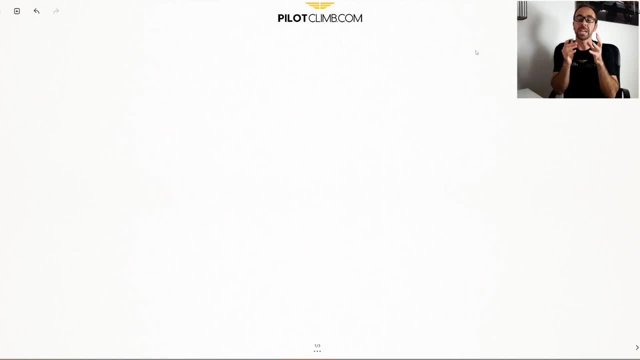 adiabatic lapse rate and the saturated adiabatic lapse rate, and I strongly recommend to watch that because in there you really understand what happens to the mass of air when it climbs, However, very quickly. the environmental lapse rate is the change in temperature with the 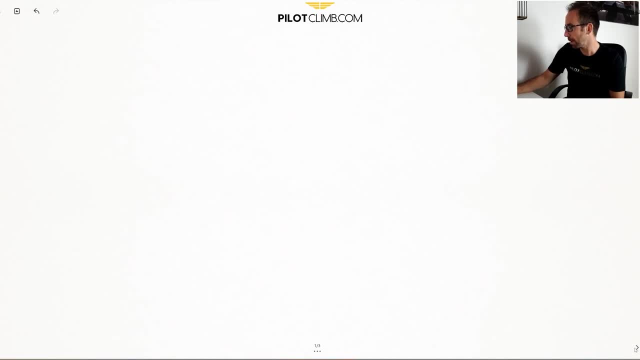 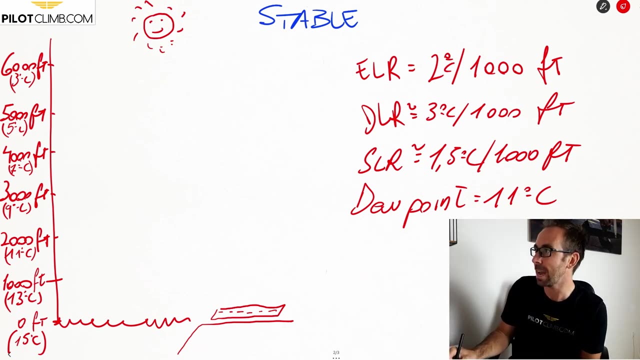 height. So if you look at the whiteboard in there again we go on the page number two and, as you can see, the environmental lapse rate, like in this case, in here is the change in temperature with the altitude According to the standard atmosphere, the environmental lapse rate, the generic atmospheric lapse rate means that the temperature will decrease every 1000 feet in elevation by 2 degrees. So if on the mean sea level the temperature is 15 degrees, what will happen is that at 1000 feet higher the temperature will be 13 degrees. 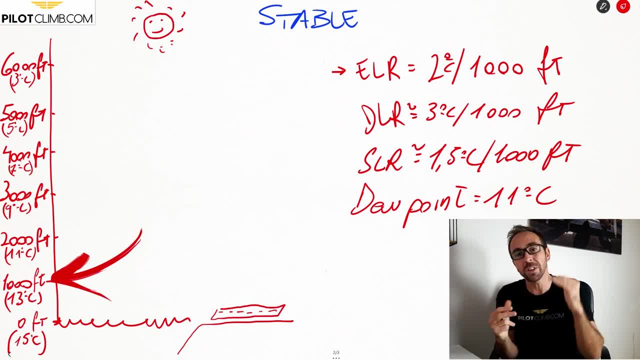 So every 1000 feet the temperature will be lower by 2 degrees. So the temperature will be lower by 2 degrees. So this is crucial to understand the atmospheric stability. Then we have the dry lapse rate, which is how much the temperature will drop, will decrease. 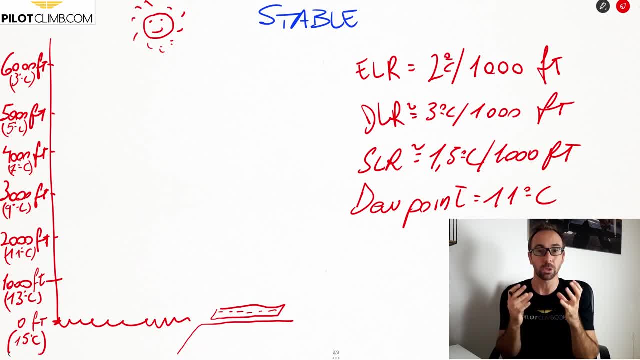 with the altitude of an air mass that is dry, that is not saturated, that is still not a cloud. Then we've got the SLR, and this is the DLR. Then we have the SLR, which is the saturated lapse rate, which is the temperature change. 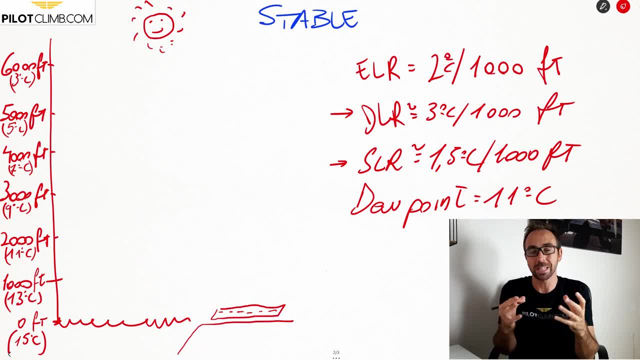 with the altitude of an air mass that is not saturated. Then we have the SLR, and this is the DLR. Then we have the SLR, which is the temperature change with the altitude of an air mass that is saturated, that gets condensate, that becomes a cloud. 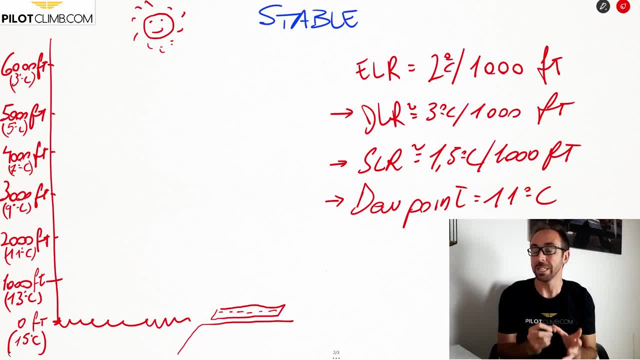 And then, lastly, we have the dew point in this slide, which is the temperature at which a mass of earth that is dry, so it's not, condensed, if you cool down the mass of earth to that temperature, that mass of earth will actually become a cloud and condensate. 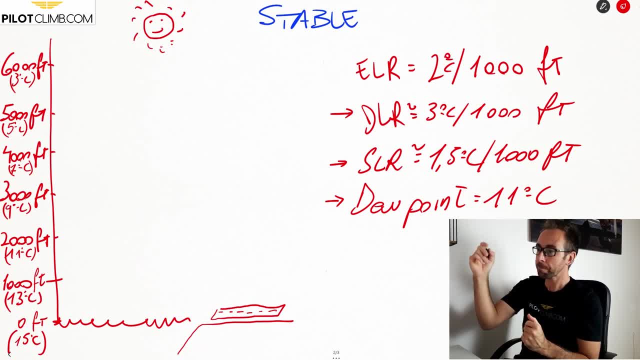 And I made a separate video where I talk about dew points. So now, in order to understand the atmospheric stability, we really need to understand what is the environmental lapse rate. What is the environmental lapse rate compared to the lapse rate of an air mass? 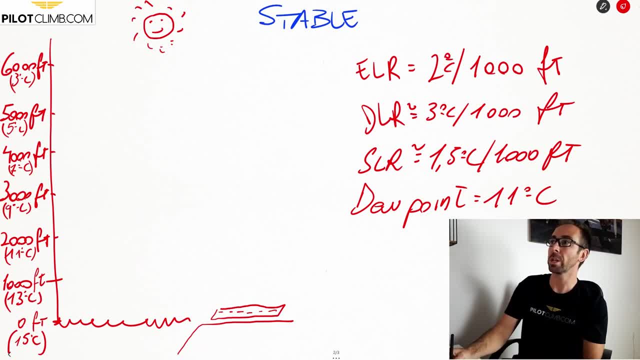 Because that is crucial. okay, Because, let's say, in this example we are talking about a stable atmosphere And, as you can see here on the left, at zero feet on the mean sea level, the temperature is 15 degrees Celsius. okay, 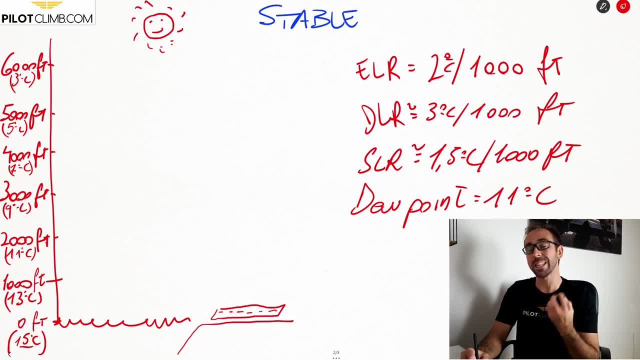 One thousand feet above, we've got 13 degrees because, according to the standard atmosphere, every thousand feet the temperature will go down by two degrees. At two thousand feet, 11 degrees and so on. Beautiful. Now let me ask you a question. 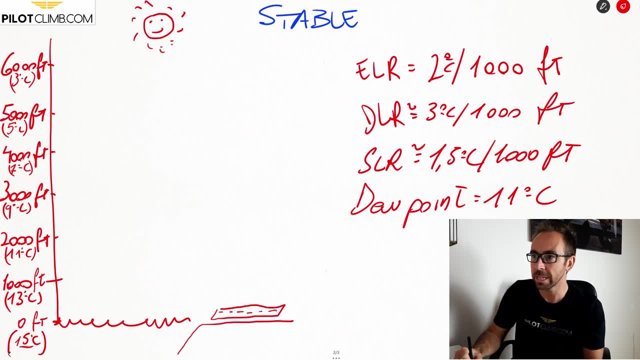 What will happen If you have a mass of air that is in here, let's say at one thousand feet. okay, Let's draw here a mass of air, just a mass of air. it's not a cloud, just a mass of air. 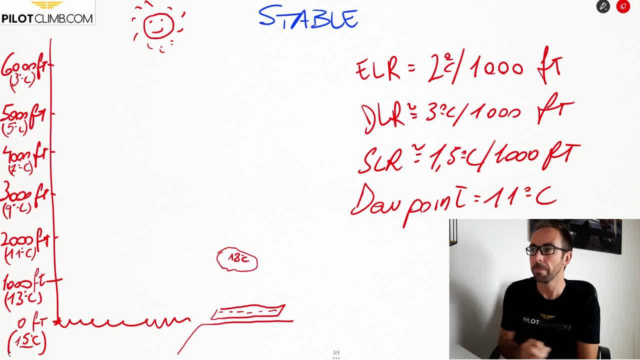 okay, That has got a temperature of 18 degrees, for example. What would happen to that mass of air, Since that mass of air is warmer compared to the surrounding air? okay, the air at one thousand feet. okay, the air that you've got in here, which is a temperature of 13 degrees. 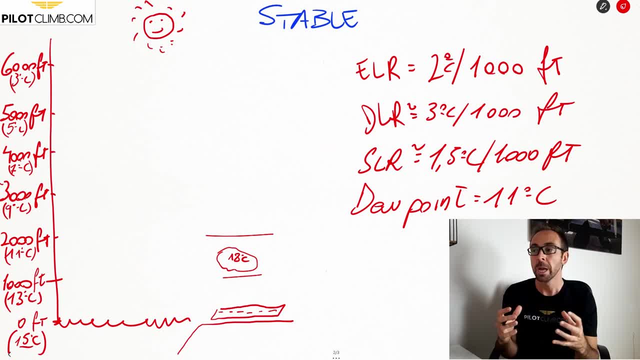 that means that the mass of air is warmer compared to the temperature that is in the air That is around it, And what will happen is this: is warmer, it's lighter. it will climb because it's lighter compared to the surrounding air. okay, 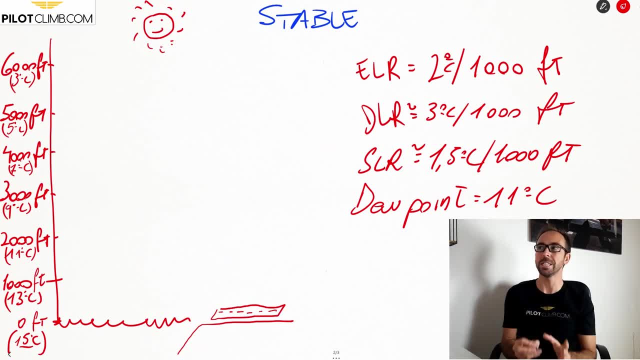 So this is crucial to understand. okay, So now let's see what happens on a stable environment On the top. there you see the sun. okay, The sun will warm up the air surface, as we explained earlier, So it will warm up the sea and the road in this case. okay, 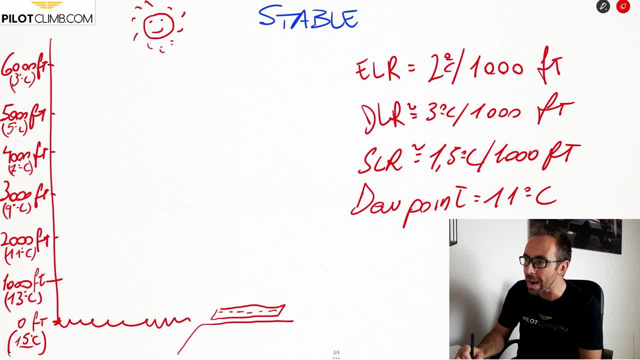 An asphalt, okay. So what will happen is that Let's say that the air on the surface okay, The air on the surface okay On top of the runway, this mass of air in here on top of the runway, will have a temperature. 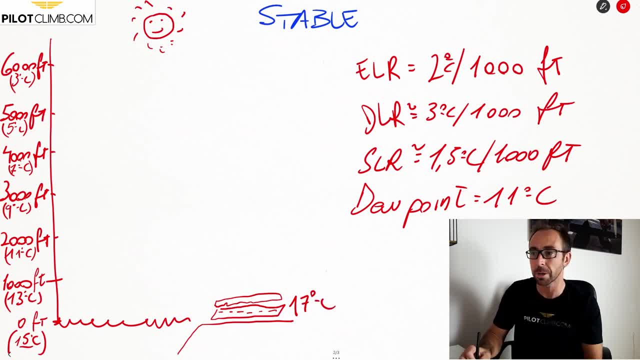 of 17 degrees Celsius, which is warmer compared to the temperature at the sea. Why? Because, as we said before, the asphalt gets warmer quicker. okay, So, since the mass of air at the mean sea level is 17 degrees, what will happen is that it 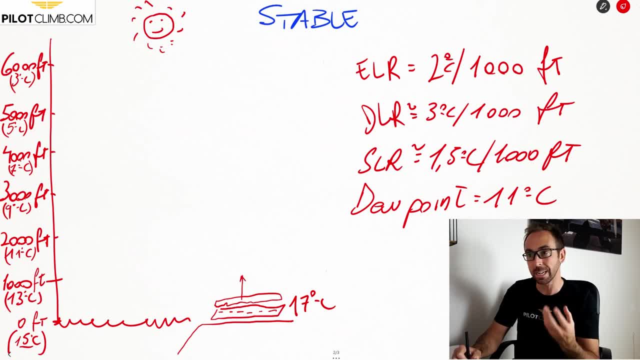 will start climbing because it's lighter. it's less dense than it does. it's lighter And since this mass of air is dry, it will go. the temperature will decrease as well, and it will decrease, And at a rate of 3 degrees per thousand feet. thus it will get to the first 1,000 feet. 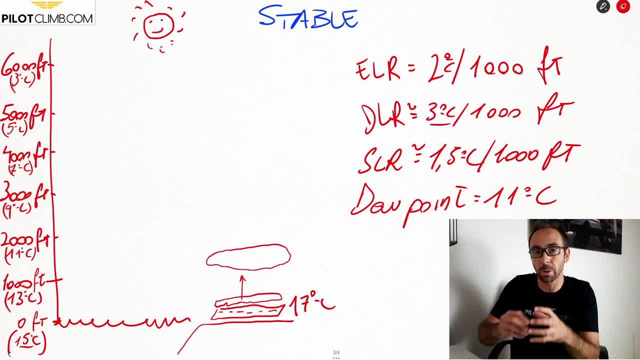 So it will be here. this mass of air will be slightly bigger because as it climbs, it expands, okay, And it will have a temperature of 14 degrees Celsius. okay, So, as you can see, at 1,000 feet, okay, this mass of air composition will have 14 degrees. 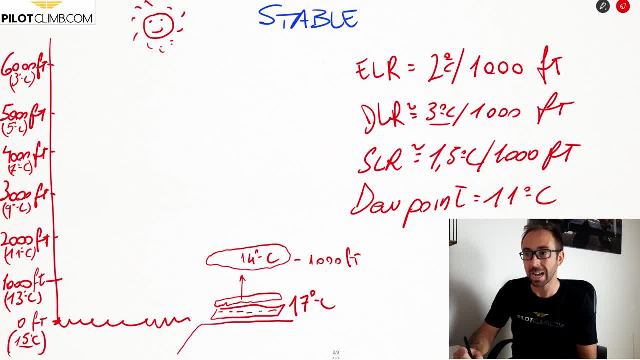 at 1,000 feet, However, the temperature around this mass of air at 1,000 feet will be 15 degrees Celsius. Okay, So at 1,000 feet it will be 13 degrees. Thus, as you can see in here, this is crucial to understand, guys- is that this mass of 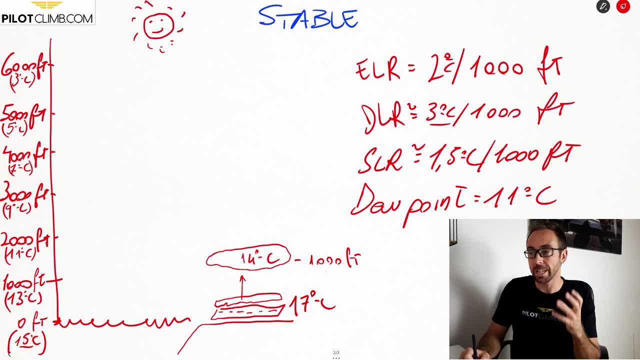 air will be still warmer compared to the outside air. Thus being warmer, that means that it will keep climbing. okay, Now let's say that the new point of this mass of air is 11 degrees. okay, So, once that this mass of air that we're talking about before gets to 11 degrees, it will condense. 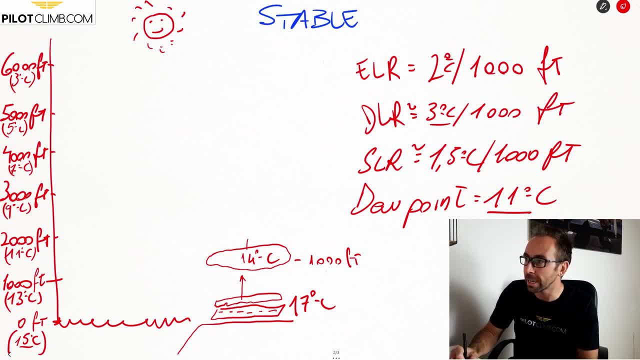 and become a cloud. Thus, let's say it climbs, It still climbs another 1,000 feet. It will reach the 2,000 feet mark and in there this mass of air will be bigger because it's expanding and the temperature will be 11 degrees because it's still dry and it's 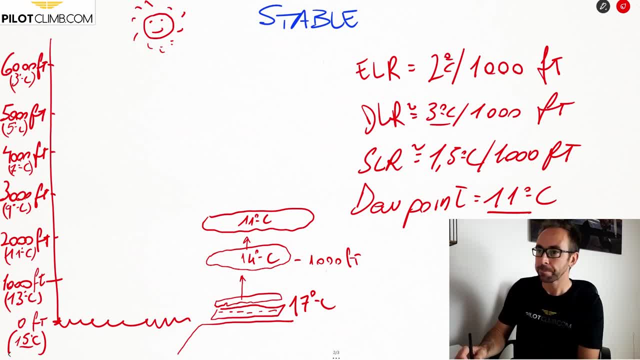 going down. The temperature is dropping by 3 degrees every 1,000 feet, As you can see in this example, at 2,000 feet, guys, this again it's crucial to understand. What will happen is that you will reach the new point. 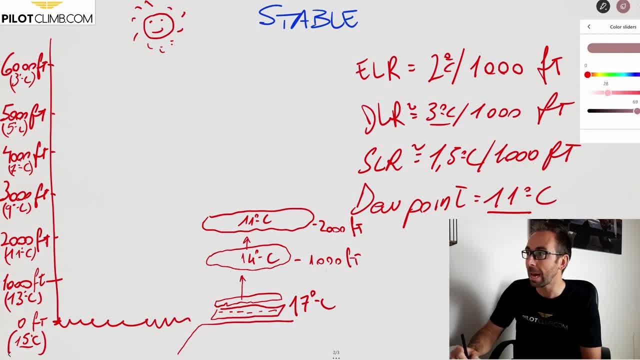 Thus, the mass of air will be a cloud, okay, will condense and be a cloud, okay. in this example, Now it's a cloud, so you can really see it visually, all right, And as you can see in here, the temperature of the mass of air, in this case, a cloud. 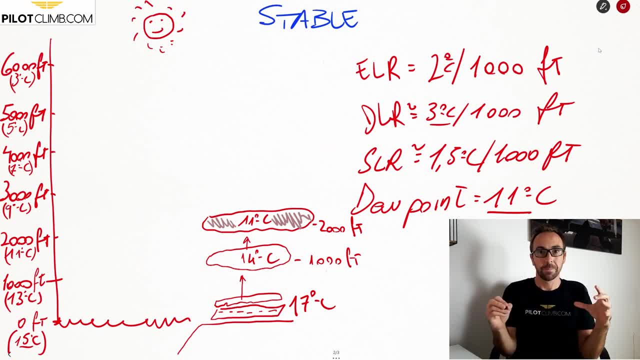 now and the temperature of the surrounding air is the same. Thus, what will happen is that, since the weight of the mass of air and the outside air temperature are the same, the mass of air will stay there, will condense and will be there, will stay. 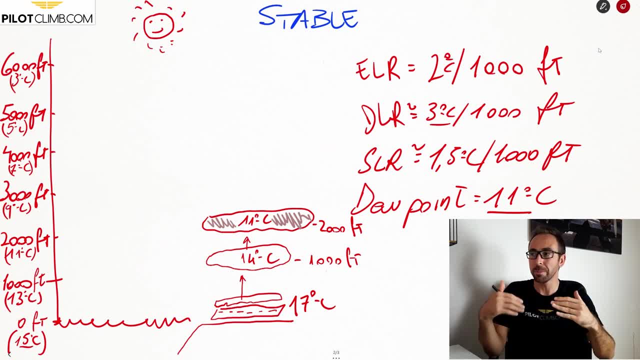 there, Boom. Okay, You won't have any other vertical movement because the temperature is the same. the mass of air temperature, The temperature of the outside air temperature is the same. Thus, once the mass of air reaches condensation, it reaches the temperature of the outside air. 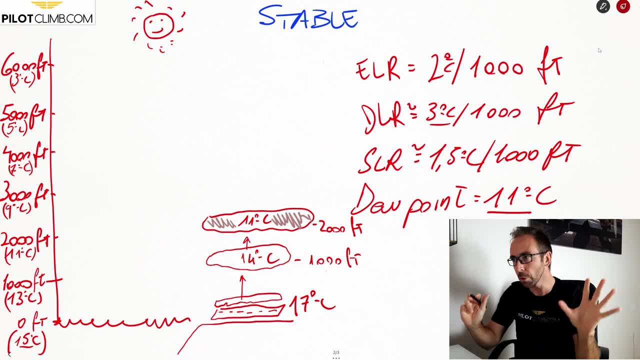 it will stay there. It condenses. it will stay there. okay, Beautiful, This is a stable environment. okay, As you can see, you're going to have a low, since you won't have any vertical movement of air, because the air, the temperature of the mass of air, is the same amount of the 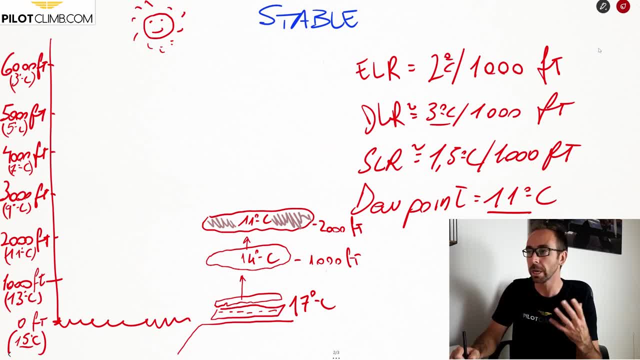 outside air. okay, you won't have any other vertical movement, okay, So you're going to have low level clouds, Like very, very thin clouds, and that's it. okay, Guys, this is very important to understand. The environmental lapse rate is two degrees every thousand feet, but this is a standard. 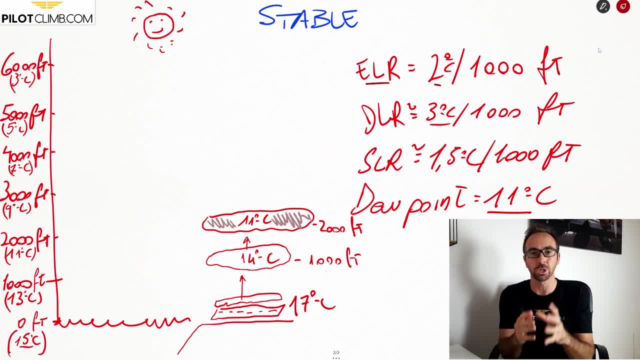 number In real life. guys. the lapse rate, they change constantly. okay, So the environmental lapse rate, the temperature change with the altitude of the atmosphere, can be one degree, or can be three, or can be five, depending on the day, but the standard. 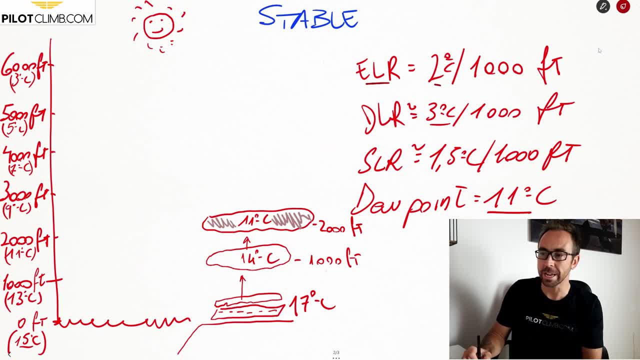 is two degrees. So let's say that another day we start at 15 degrees at the mean sea level. However, at one thousand feet, your environmental lapse rate, instead of being two degrees as per the standard one, it's going to be one degree. 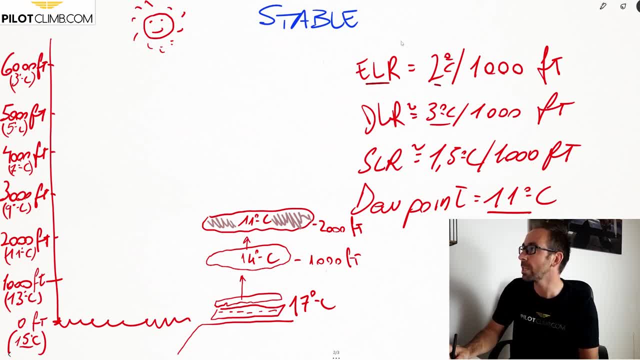 So let me make a correction in here. There we go. Let's say that now, in this example, instead of having two degrees per thousand feet, let's call it one degree, okay, And let's see what will happen to your mass of air and your atmospheric stability, okay. 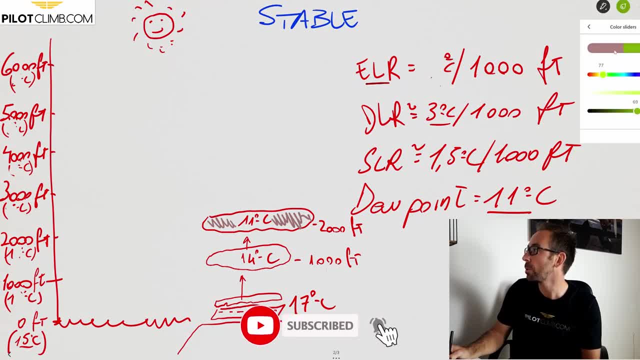 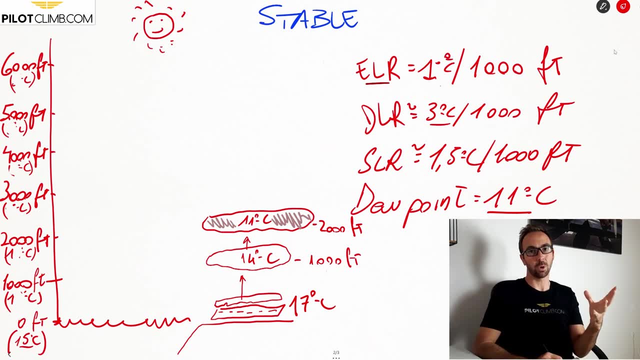 So I change the color in here. I take the red one, So that's the red one. Here we go, Beautiful. So let's say that now the environmental lapse rate is one degree only. okay, Because this is not a standard environmental lapse rate, it's one degree. 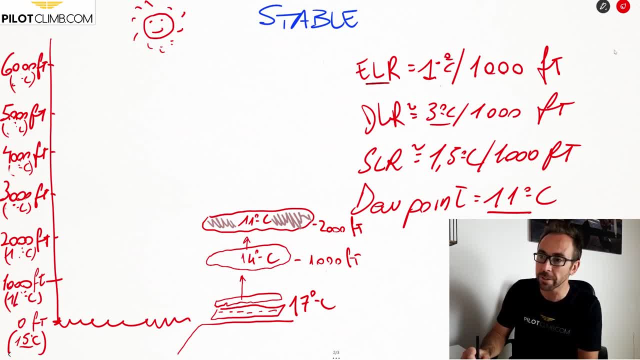 So what will happen is that, at zero feet, you're going to have 15 degrees. one thousand feet, you're going to be 14 degrees. two thousand feet, you're going to be 13 degrees. at three thousand feet, you're going to be 12,, 11,, 10, and nine degrees. okay, 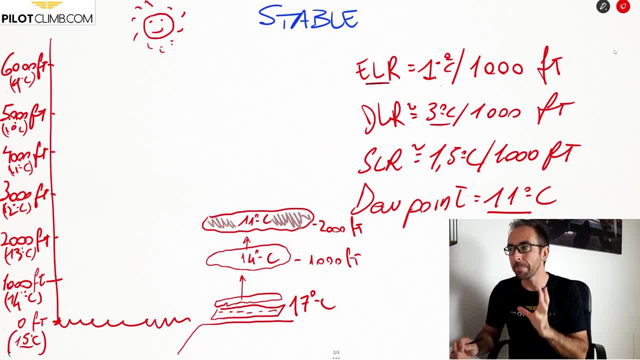 This is the outside air temperature, okay, And let's say that the mass of air, it will stay the same, So the characteristic of the mass of air won't change. okay, In order to understand, guys, because this is crucial, because in order to understand, 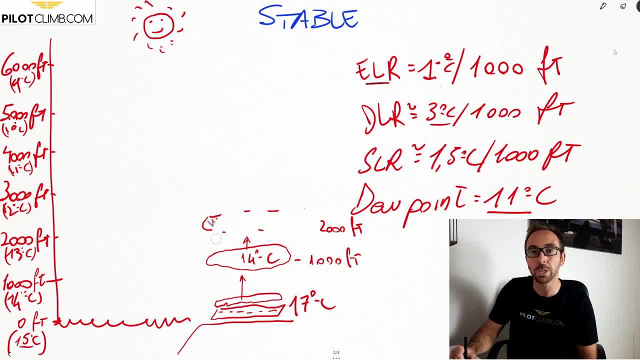 the atmospheric stability. you need to make sure that you understand that this is all about environmental lapse rate and the lapse rate of the mass of air. okay, So let's do the other example, where we talk about the, where we have an environmental lapse rate of one degree. all right? 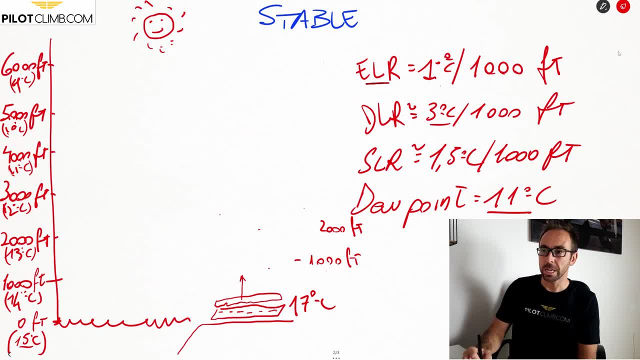 So now, beautiful. So if you come in here, guys, we start at zero feet, 15 degrees. okay, Let's see. Let's say we start at 17 degrees. thus this mass of air, the mass of air, is warmer than 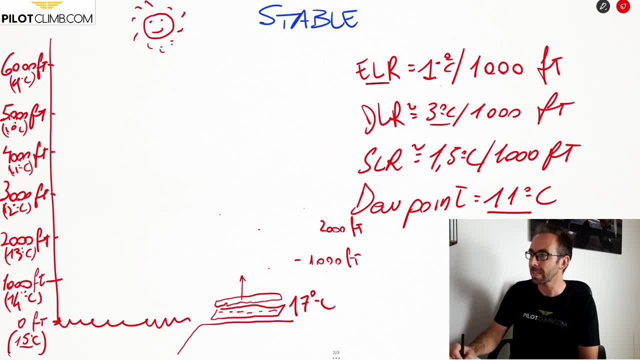 the outside air. so it will start rise. So the temperature, the dry, the mass of air will decrease its temperature by three degrees every thousand feet. thus it will get to the first one thousand feet and we'll have. it's going to be in here, and 17 minus three is 14 degrees. 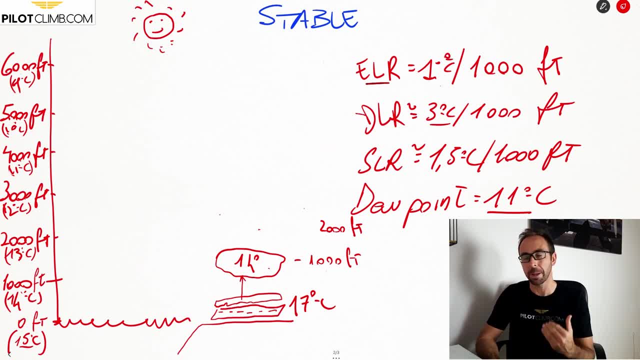 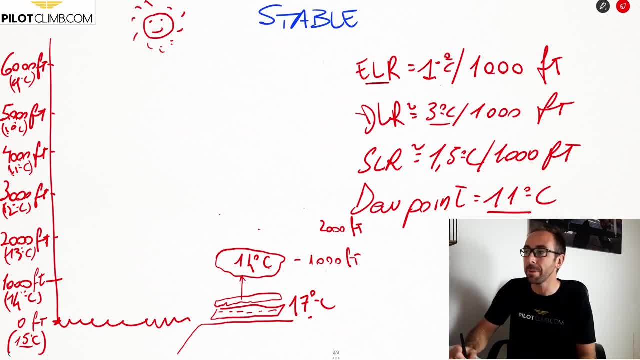 It will not even reach its due point because it cannot climb anymore and reach the 11 degrees needed to condensate. okay, So in this case, as you can see, it's stable because the vertical movement of the mass of air will be subcutaneous. 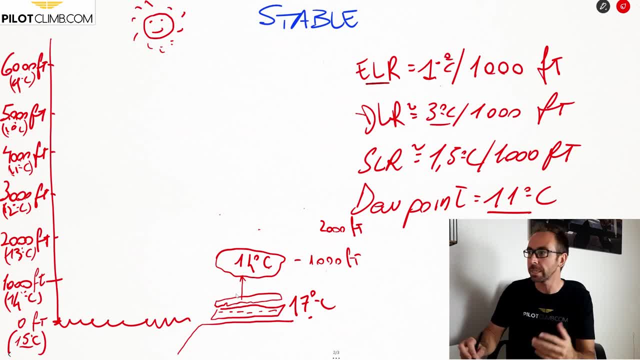 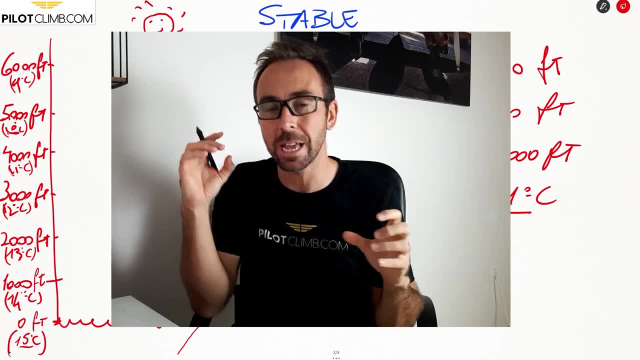 It will be suppressed, almost okay, So it won't go anywhere there, all right. So this is very important to understand guys. Stability and unstability of the atmosphere: it's all about environmental lapse rate and the lapse rate of the air mass. 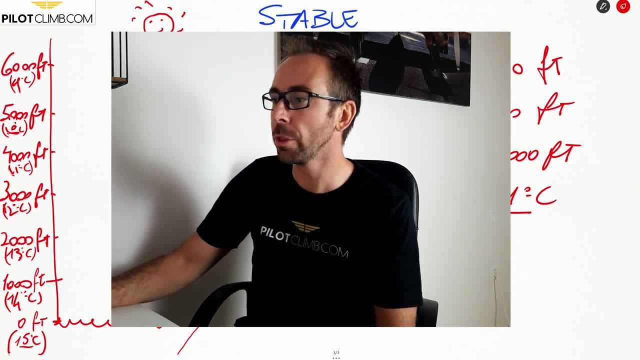 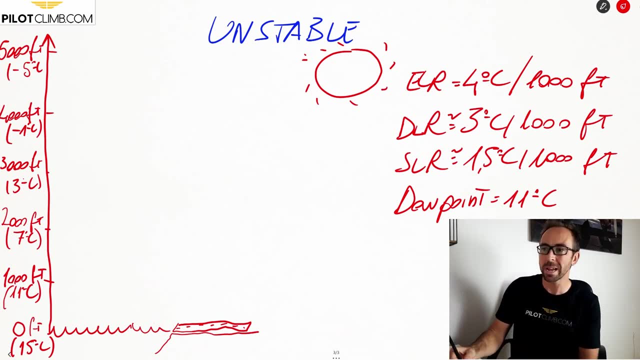 Right, let's make another example, If you go to the next page. okay, that is an unstable atmosphere, okay, So let's analyze the environmental lapse rate. The environmental lapse rate: okay, the general temperature change with the altitude is four. 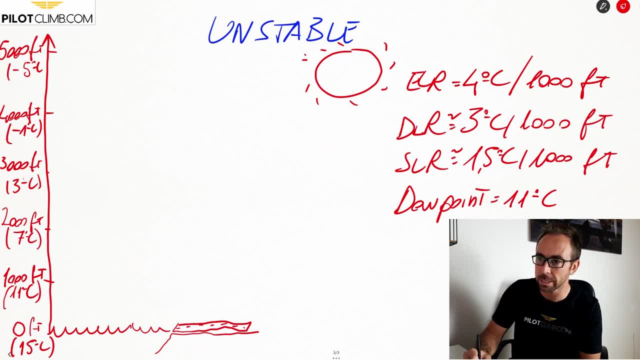 degrees Celsius. okay, As you can see in here, at zero feet on the missile level, at 50 degrees, 1,000 feet above, we have 11 degrees. Why? Because the environmental lapse rate is four degrees per 1,000 feet. 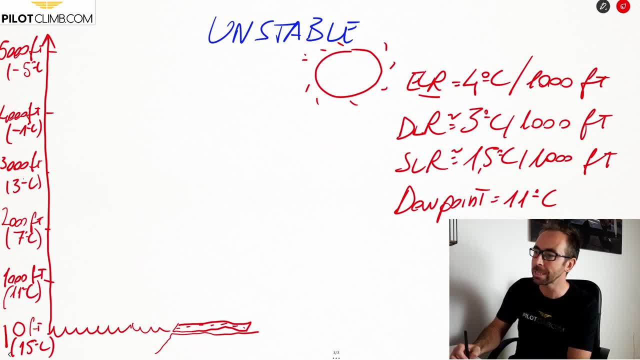 So this is a non-standard environmental lapse rate. okay, So let's make the same example. So let's start with. the sun will warm up the sea and warm up the runway, thus the mass of air that is on top of the runway. let's say that we just follow the example, as before. 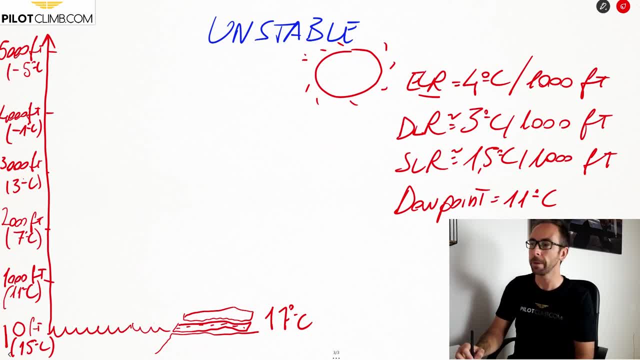 okay, And this mass of air will start at 17 degrees. okay, Beautiful, Let's have a look. We climb, because this is warmer than the 15 degrees. okay, It will climb and it will get to the first 1,000 feet, this mass of air, okay. 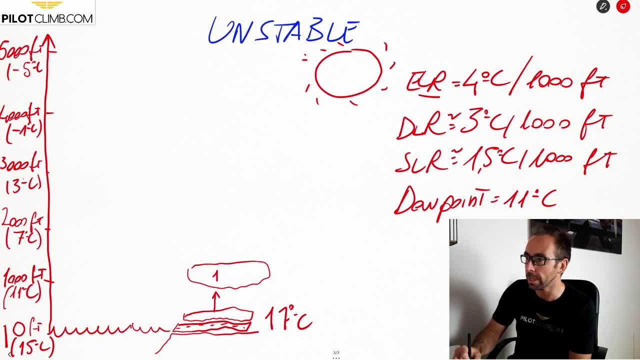 It will be in here and it's going to have a temperature of 14 degrees. Thus, if you compare the temperature of the mass of air with the surrounding air, it's warmer. Thus it's still lighter. It will climb another 1,000 feet, okay. 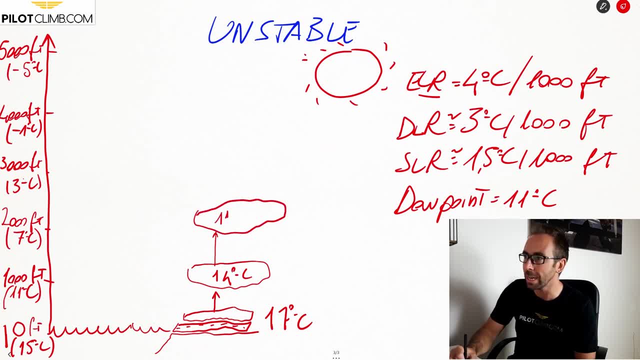 And then at 2,000 feet, This mass of air will get to the 11 degrees Celsius. If you compare to the 2,000 feet temperature of the outside air, it's going to be 7, thus the mass of air is still warmer and lighter. 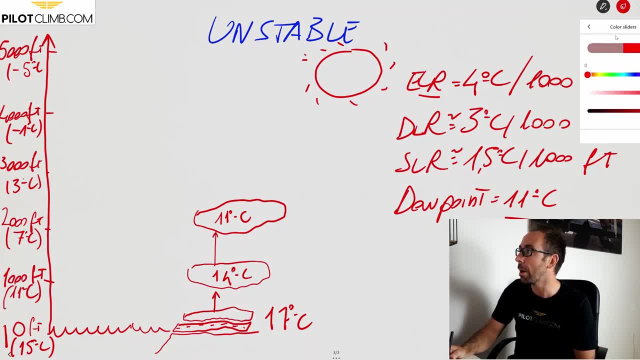 But now, since we are 11 degrees, we actually reached our condensation, our dew point. Thus, this mass of air will change. okay, It will become a cloud now. So, now we've got a cloud, The clouds will climb. 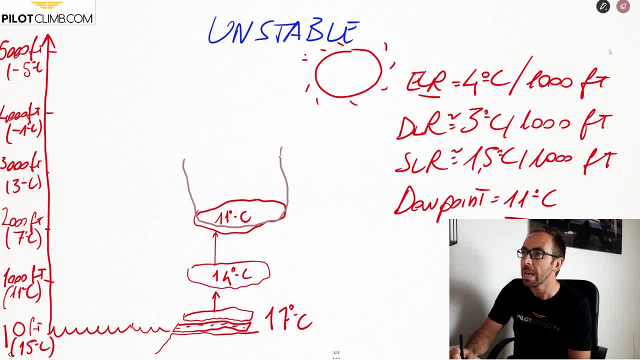 We start to form a cloud, okay, And we'll get to the 3,000 feet. okay, At the 3,000 feet, At the 3,000 feet, the temperature of the cloud will be 11 minus. So now we need to use the SLR because the cloud is formatted, so we are saturated, okay. 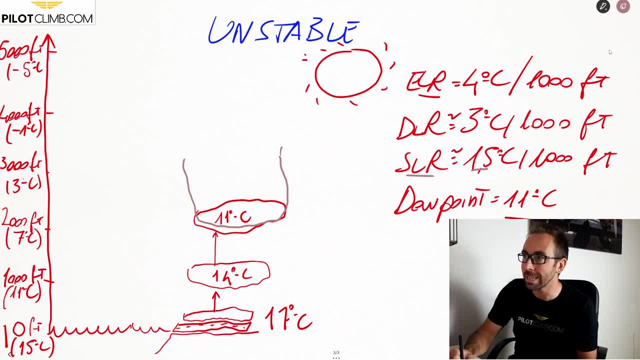 We are following this saturated lapse rate. So let's say the cloud will climb to the 3,000 feet. okay, And what is the temperature of the cloud at 3,000 feet? Let's call it 2 degrees. So 11 minus 2 is 9 degrees. okay, 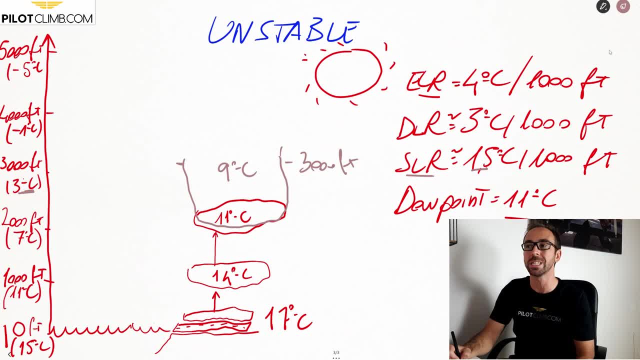 9 degrees Celsius. If you compare to the outside air temperature, it's 3 degrees. Thus, the cloud is still warmer. Okay, It's still warmer. So what will happen is that we keep climbing to the 4,000 feet and another 2 degrees colder. 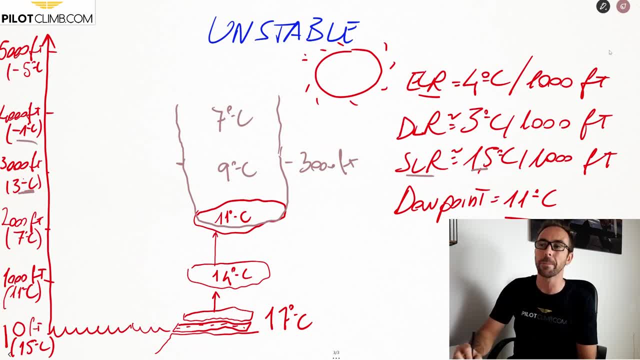 so the cloud will have 7 degrees and the outside air temperature will be minus 1.. Thus it's still warmer. So we'll keep climbing, because the air is always warmer and lighter. And that is the difference, because on a stable atmosphere the air mass at some point will. 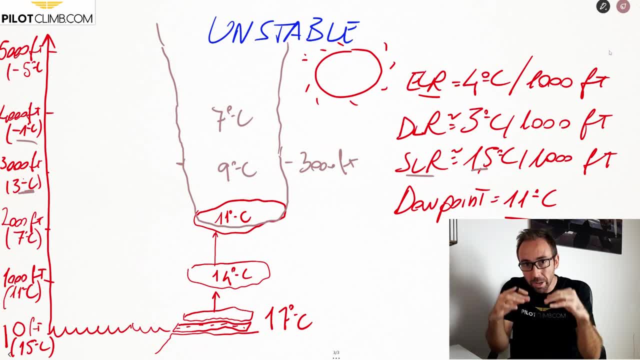 become heavier and colder. Thus it will stay there or will go down In the An unstable atmosphere. The mass over will be always warmer and lighter, Thus it will climb. It will reach the new point, it will become a cloud, and then it will keep climbing, condensated.